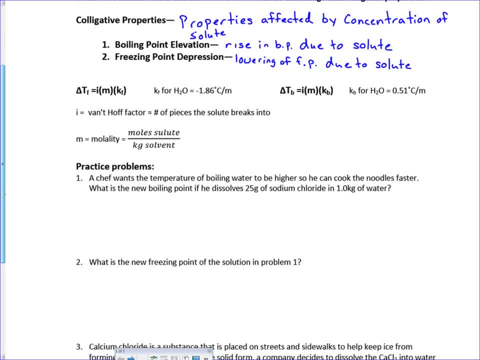 of pieces that something's going to break into. And so really what you're thinking about here with the Van't Hoff factor is, if it's ionic, it's going to break into however many atoms or any ions. So NaCl would break into two. 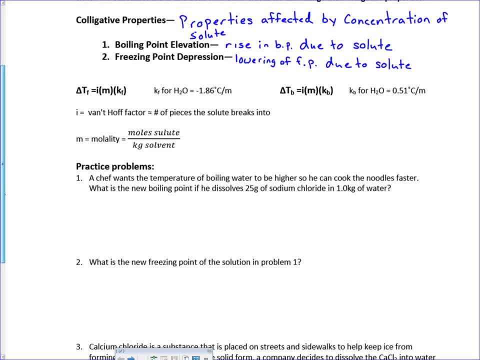 pieces. CaCl2 would break into three pieces, AlI3 would break into four pieces, things like that, And so however many pieces there are for the ion, it's going to break into it For something that's covalent, for something that just has non-metals in it: the Van't. Hoff factor is going to be one, And so it's sort of important that you understand that. Okay, so the Van't Hoff factor is going to be one, And so it's sort of important that you understand that. Okay, so the Van't Hoff factor is going to be one, And so it's sort of important that you 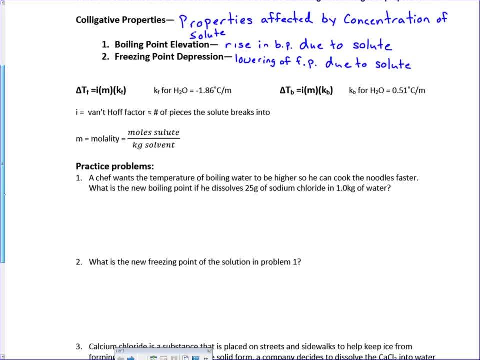 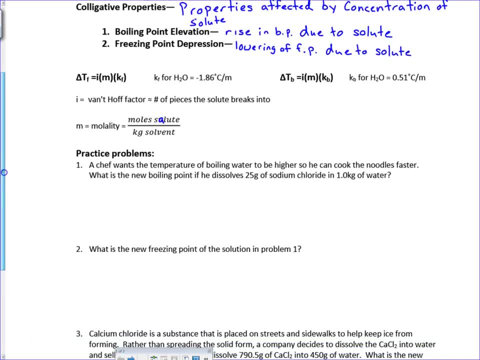 understand how to get that Van't Hoff factor Molality, That's the moles of the solute over the kilograms of solvent. So this should be an A here. All right, so we're going to go through and do a few practice problems here and then. 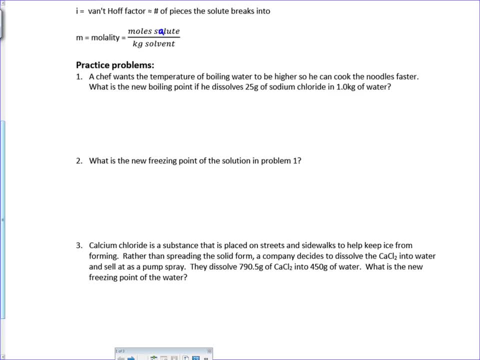 I'll go through the main sheet. So this first one here starts offit says you've got sodium chloride And we're wondering if the chef's adding this salt or sodium chloride to a a pot of water, how much faster it is going to boil or, sorry, how much hotter it's going. 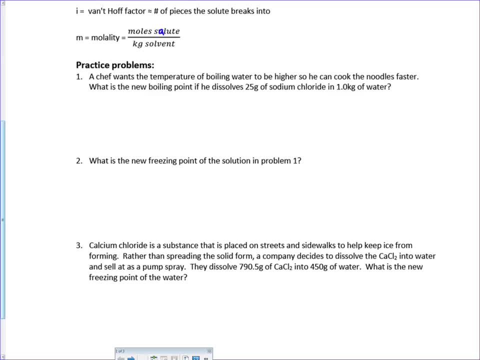 to boil, And so what we get here, then you have to realize if it's NaCl, if it's just normal salt, then the Van't Hoff factor is going to equal 2. That will come into play later. We start with 25 grams. We need to get to molality, which means we need to find 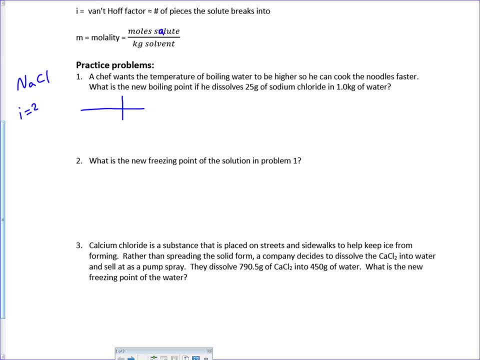 the moles of salt. To do that we need to go from grams to moles, using the molar mass from the periodic table. So we start 25.0 grams of NaCl. Then if you look up on the periodic table you can find 58.44 grams in one mole. You multiply those, you get 0.428. 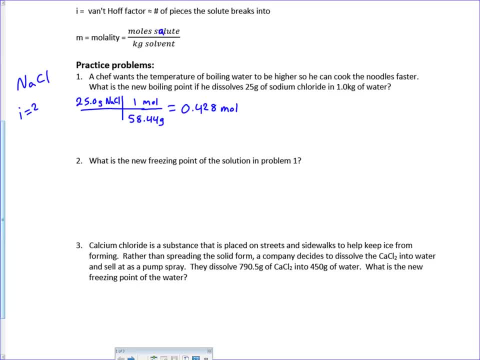 moles. Alright, now we can calculate molality. Molality is the moles of the solute, so that's that 0.428.. Over kilograms of the solvent, in this case, it's just 1.0.. That ends up giving us 0.428. 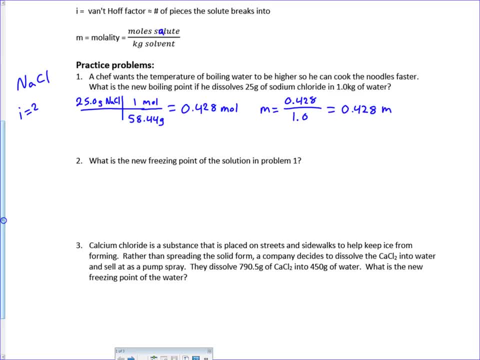 again, because it was just divided by 1. Now we're in units of molal. So now we're going to calculate the change in boiling temperature. For that we say: change in boiling temperature equals I times molality, times your boiling point, constant Kf. 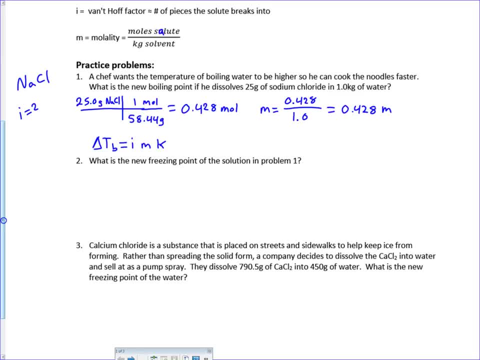 Whoops, Kb. Alright, so now we'll multiply them. That's 2.. The molality is 0.428.. And then the constant there is 0.51.. And this is for water. So every time you're using water, 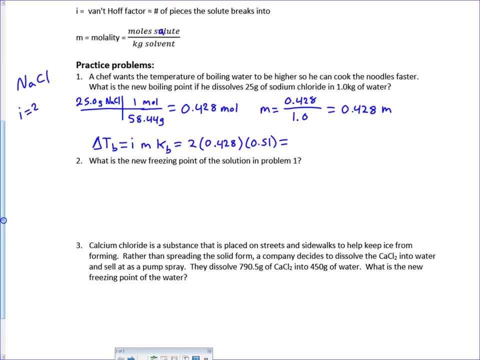 as your solvent. that's what it will be. You go through, you get 0.437 degrees Celsius. Now, this isn't your final answer. This is just telling you how much the boiling point is going to change. The normal boiling point for water is 100.. And so if it's going up, 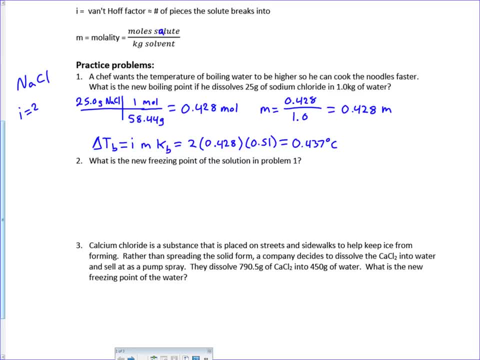 it's elevated, it's boiling point elevation. then we're elevating it by 0.437 degrees Celsius, which means our new boiling point, our new boiling temperature is going to be 100.437.. So we're just adding 100 to it because the normal boiling point is at 100 and we're changing. 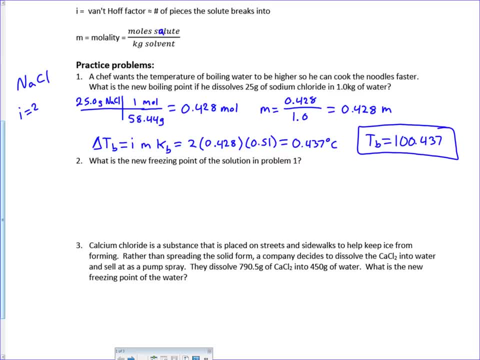 it by going up by 0.437.. And we should have degrees Celsius here. Number two: it says freezing point, same solution, And so we don't have to do all the calculations that we did originally, because that was just to get molality, So we can jump right to delta. 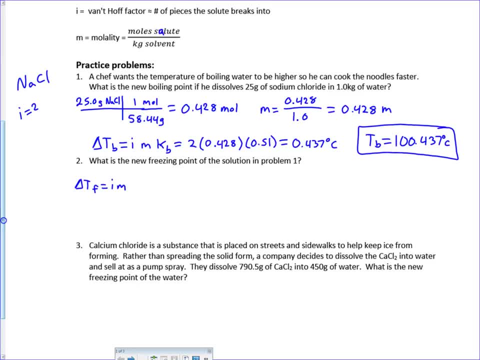 Tf equals I times M times Kf, which equals 2 times again, 0.428 times. your boiling point is our Kf. That's negative 1.86.. We multiply all those together, we get negative 1.59 degrees. 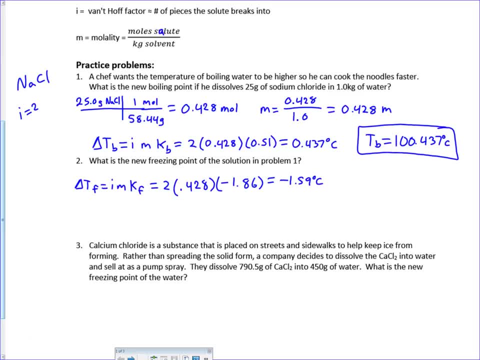 Celsius. All right, so this is the change in temperature. It's going down. The freezing temperature is going down by 1.59.. Now the normal temperature is 0. And so if we're at 0 and then we go down 1.59, we actually end up at negative 1.59.. So it seems like it's the same number. 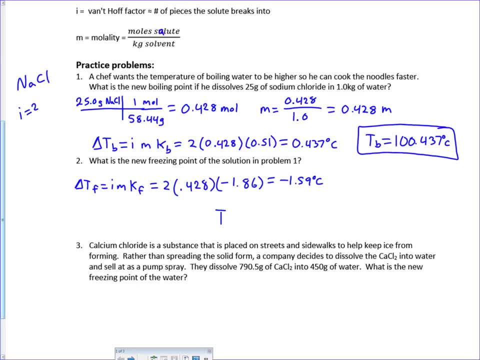 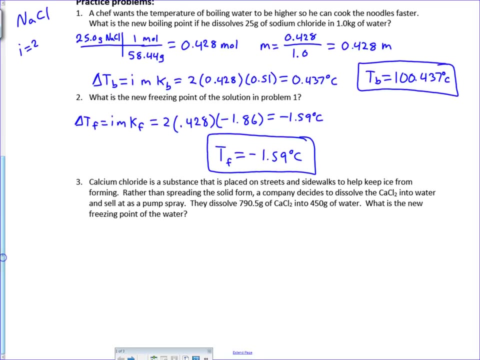 here, but that's just because the freezing point for water is 0. And if you change from 0, you're going to get whatever number that changes. So, yeah, it's negative 1.59 degrees Celsius. Problem number three here: calcium chloride substance placed on the street. So this is. 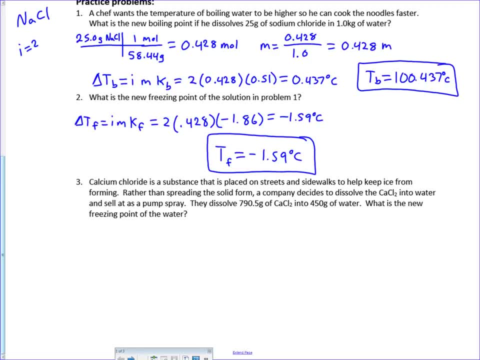 what you're using to melt normal ice on the sidewalk. It's what you go and buy at the store to melt ice. It says that they're going to put it in a spray pump here, And this is It's asking how much it changes the freezing point of water. 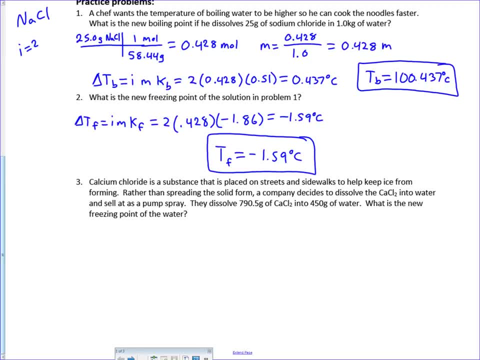 actually rather what the new freezing point would be. So our substance that we're talking about here is CaCl2, which is calcium chloride. The Vantoff factor for that one is 3.. And so we're going to do the same sort of steps as we did before. 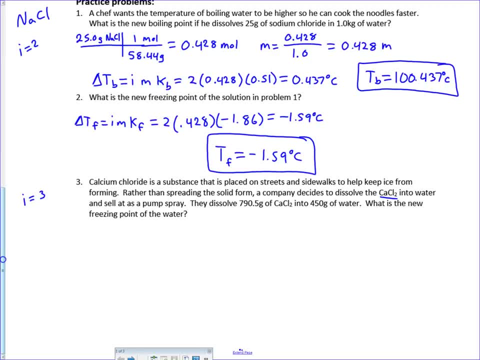 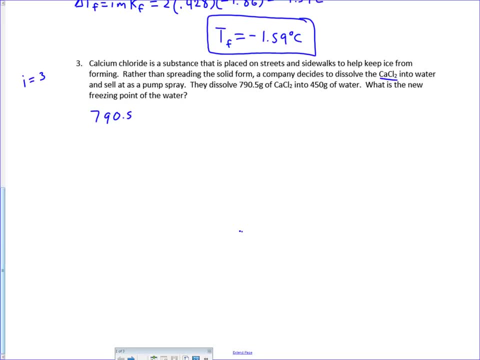 We start off with the mass that they gave us. So we've got 790.5 grams of CaCl2.. If you look up on the periodic table, you can find the mass of CaCl2.. It's 110.98 grams in one mole. 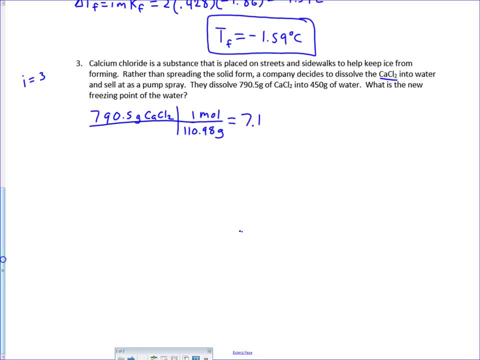 Go through, calculate that you get 7.12 moles. We're going to plug that into the molality equation. So molality equals 7.12 moles over 0.450 kilograms. Notice, here it was given in grams. 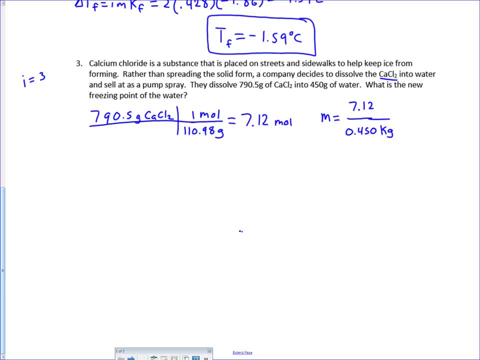 I had to convert it to kilograms because that's what the molality equation says. So then you calculate that you get 15.8 molal for the concentration there. So then we know: change in boiling temperature Or freezing temperature equals I times M times the freezing point, constant. 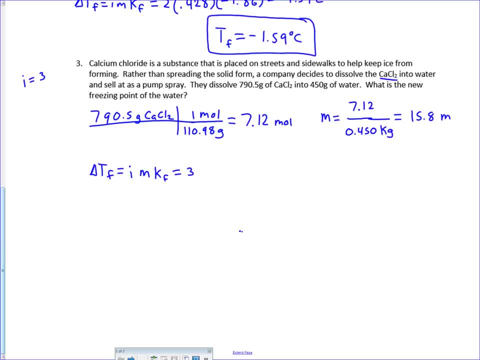 And then Vantoff factor I said is 3, because CaCl2, calcium chloride, is an ionic substance. It's going to split into three pieces 3 times 15.8, times negative 1.86.. That's 6.. 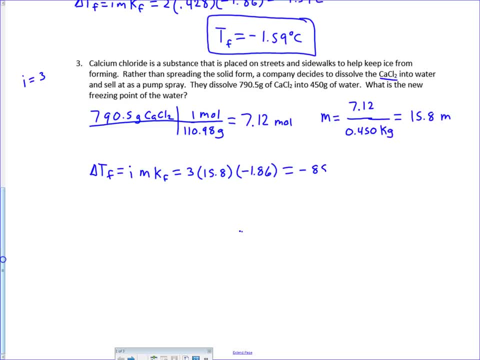 All right, multiply those together, You get negative 88.16 degrees Celsius, All right. and then for this one again, it's freezing point. This is the change in temperature. The normal is 0. So your freezing temperature is going to equal negative 88.16 degrees Celsius. 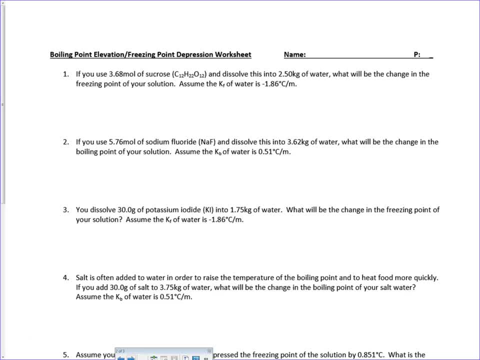 On to the next page here. So quite a few problems. It starts off pretty easy, though. We're given just moles here and kilograms, So you can calculate molality right away. You don't have to start with the grams, And so we know molality is going to equal your moles of your solute. 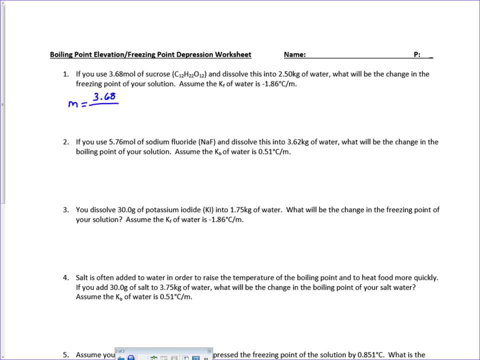 That's 3.68 moles. over your kilograms of the solvent, That's 2.5, which is going to give us 1.47 molal. Then we're going to plug it into the delta T f equation. So we know the freezing temperature here is going to change by i times m, times kf. 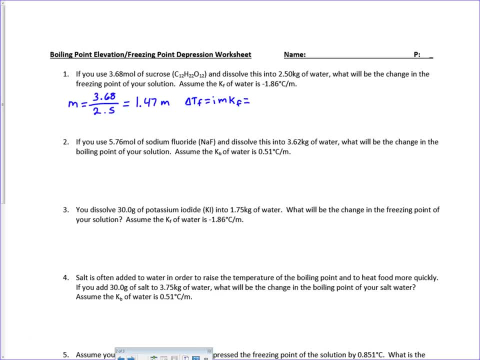 i, in this case, This is sucrose, if you see the formula there: C12H22O12.. Those ones are that's all covalent. okay, It's all nonmetals, And so this one's only going to split into moles. 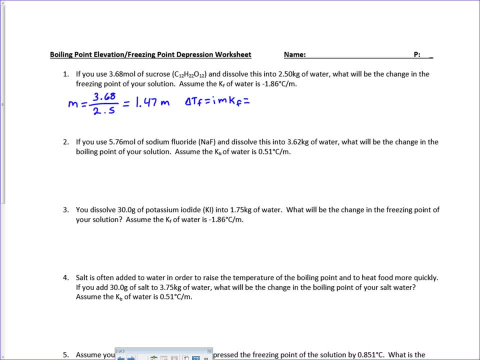 So we're going to plug it into the delta T- f equation. It's going to split into one piece or it's going to stay as one piece, however you interpret that, And so our Van't Hoff factor is 1.. The molality here is 1.47.. 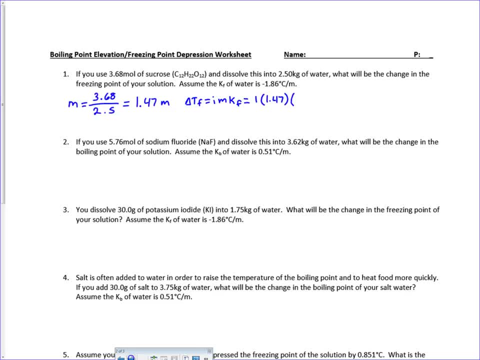 And the freezing point, depression constant, is negative 1.86.. So we go through and we multiply all that out, We get negative 2.73 degrees Celsius. Okay, so then, If we're doing this, we know that our freezing temperature 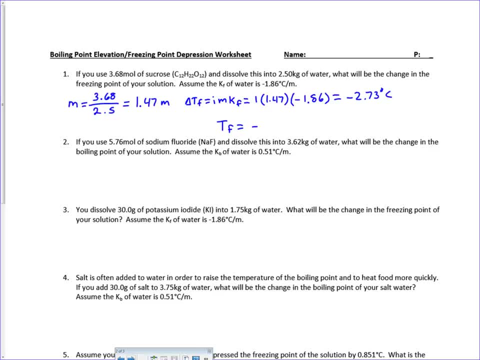 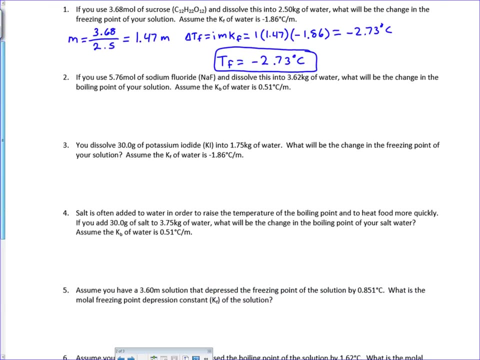 our new freezing temperature again, because it's normally zero and it's changing by negative 2.73, is going to be negative 2.73 degrees Celsius. Problem two: it says you got 5.76 moles of sodium fluoride. 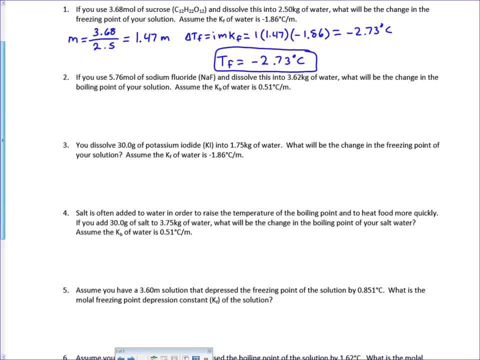 It's dissolved in 3.62 kilograms of water And it's asking what the change in the boiling point will be. So this one here, our Van't Hoff factor, is 2 because it's sodium fluoride. NaF is an ionic substance. 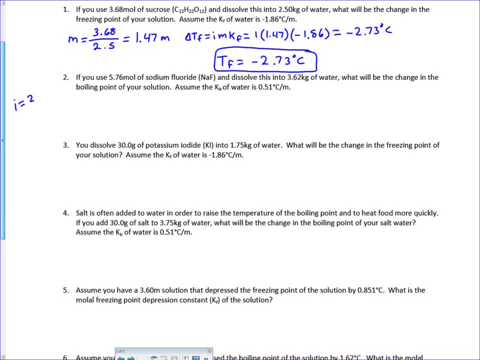 It's going to split into an Na atom and an F atom. So we're going to start here and say: the molality equals our moles 5.76, over our kilograms 3.62.. You divide those, You get 1.59.. 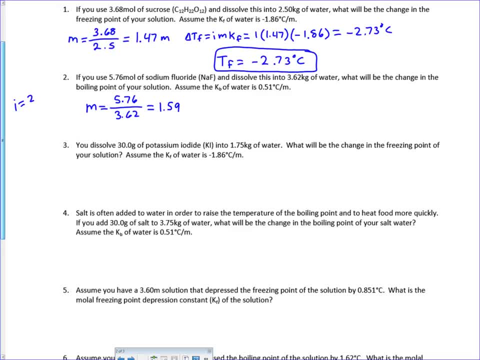 1.59.. Then we have our change in boiling. Our change in boiling temperature equals I times M times our constant for boiling, which equals 2 times 1.59 times 0.51.. If you multiply all those out, you get 1.62 degrees Celsius. 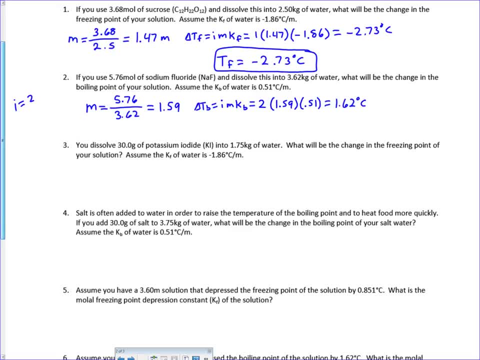 Now this is the change in temperature. Our normal boiling temperature is 100.. So here our temperature for boiling is going to equal 101.62.. So normally it's 100.. It changes by 1.62.. So we end up 101.62.. 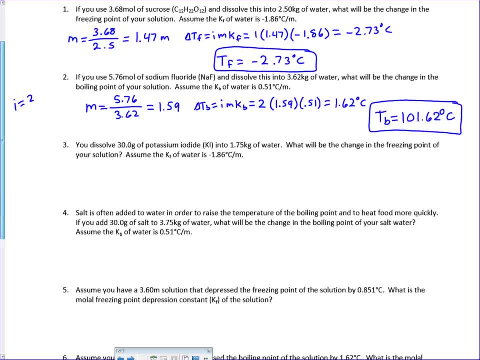 It's going to go up by 1.62 degrees Celsius from the normal Number 3. here we've got potassium iodide. Potassium iodide is ionic, So our I here is going to split into one potassium and one iodide. 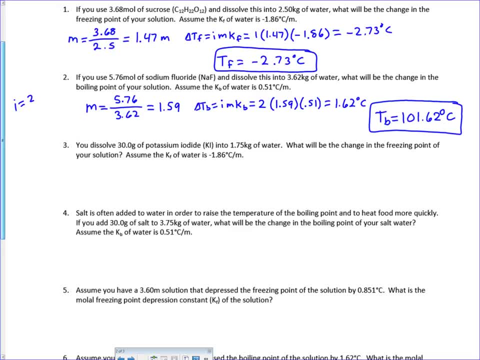 So our I is 2.. We've got 30 grams here. it's given us. We've got to convert that to 1.62.. So we're going to split that into 1.62.. So our I is 2.. 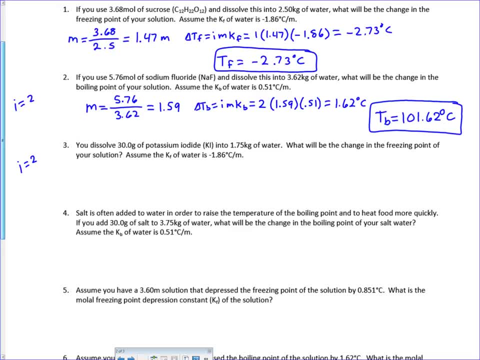 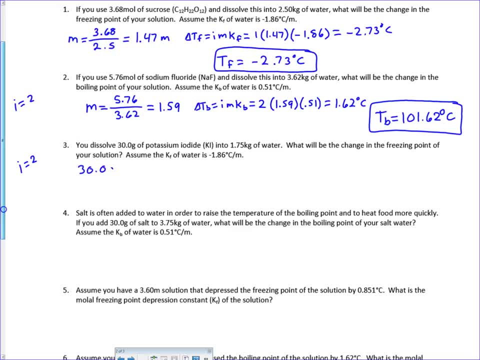 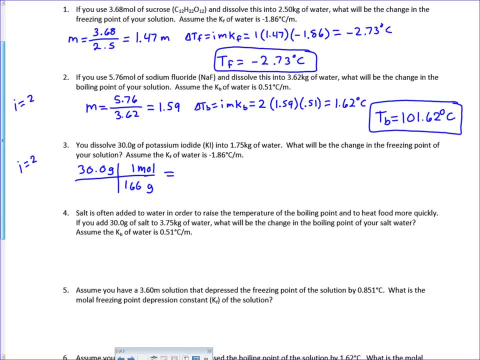 You multiply those, You multiply those, You get 0.181.. You get 0.181.. You get 0.181.. For your number of moles, For your number of moles, For your number of moles, And then we'll have our molality. 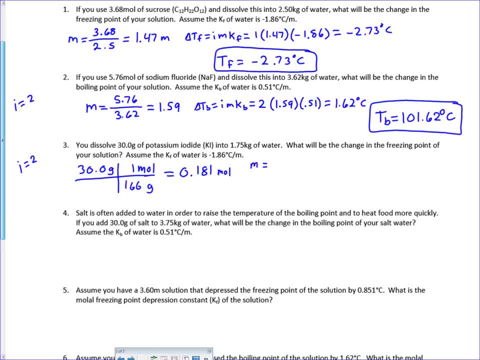 And then we'll have our molality equals 0.181, equals 0.181, equals 0.181 over 1.75, over 1.75, because it said 1.75 kilograms, You divide those, You get 0.103. 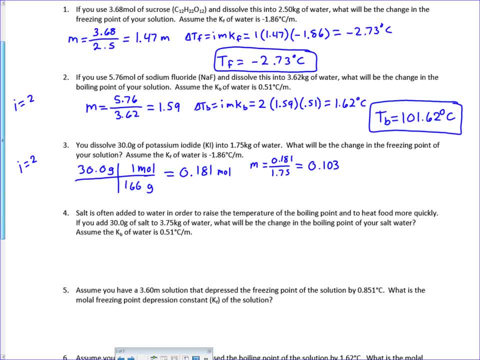 You divide those, You get 0.103. Then we know the change in the freezing temperature. Then we know the change in the freezing temperature equals our Van't Hoff factor, equals our Van't Hoff factor, which is going to be 2 times our molality. 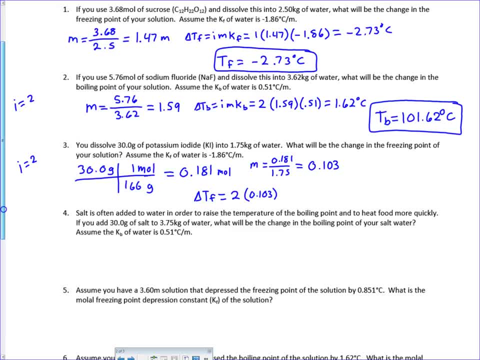 which is going to be 2 times our molality, 0.103 times the freezing point, constant times the freezing point, constant negative 1.86. Multiply all those together you get negative 0.383. you get negative 0.383 degrees Celsius, and so that means our final freezing temperature. 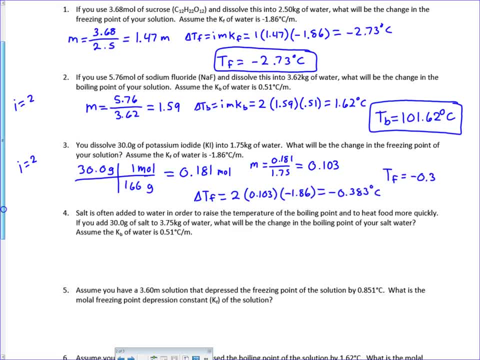 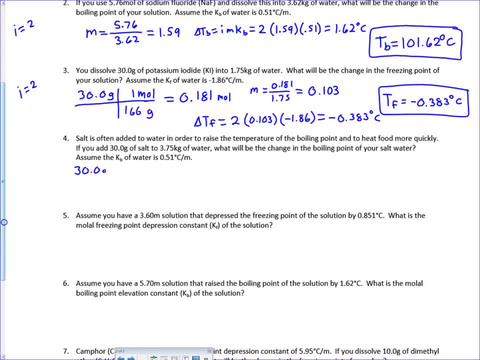 So we start here. 30.0 grams of NaCl- Very similar to the last problem In this case. 58.44 is the molar mass. is the molar mass, Multiply those, you get 0.513 moles, 0.513 moles. 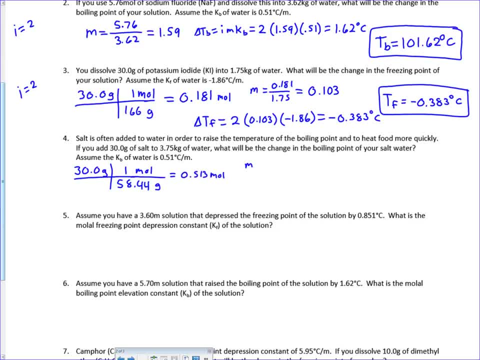 Our molality, then, is going to equal 0.513, is going to equal 0.513 divided by the kilograms 3.75, 3.75, and you get 0.137, 3.75 molal, molal, molal, molal. 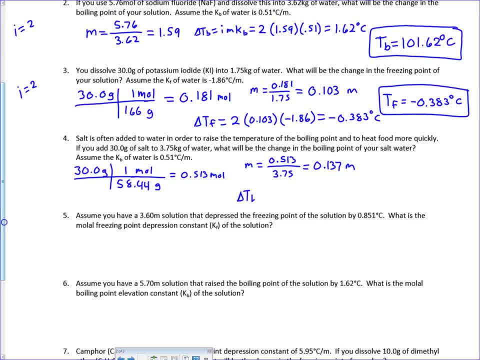 molal. Then next step here We're going to say change in boiling temperature is going to equal. I times the molality times your boiling point constant, which equals 2 times 0.137, and we get for that 0.140 degrees Celsius. Normal boiling point for water is 100,. 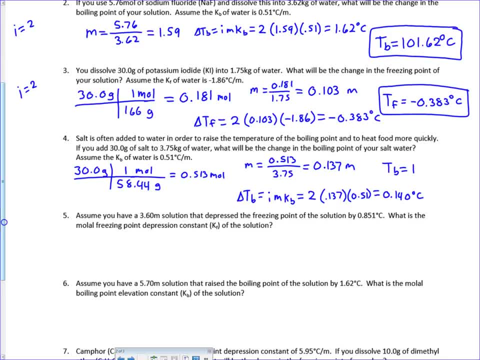 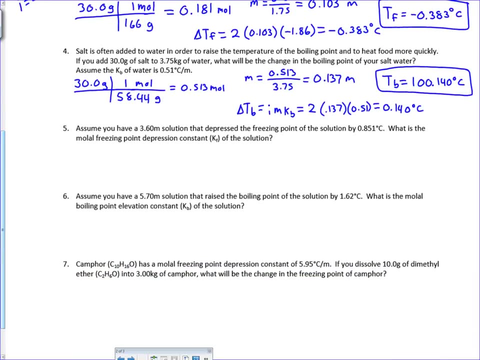 so our final boiling temperature is going to equal 100, and then it changed by 0.140,, so 100.140 degrees Celsius, Number five. so this one says we've got a 3.6 mol-al solution. it wants us to calculate Kf. 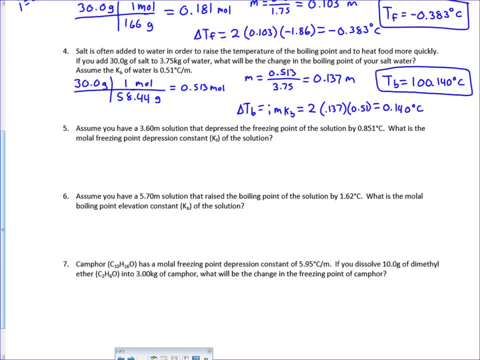 it tells us the freezing point was depressed by 0.851 degrees Celsius. On this one I didn't tell you in the problem, but you should assume I equals 1, because it doesn't tell you what the solute is, so you don't know what it would be. 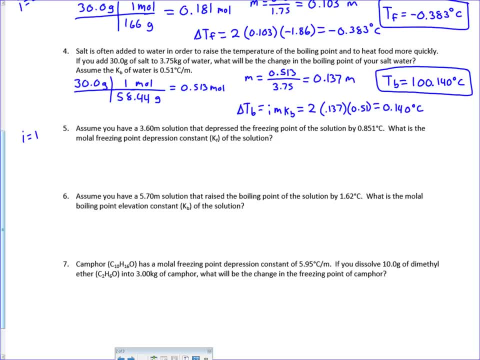 so we're going to say I equals 1.. So you just plug this in: change in freezing temperature equals I times M times Kf, and so the things that we know, we know the change in freezing temperature is 0.851,. 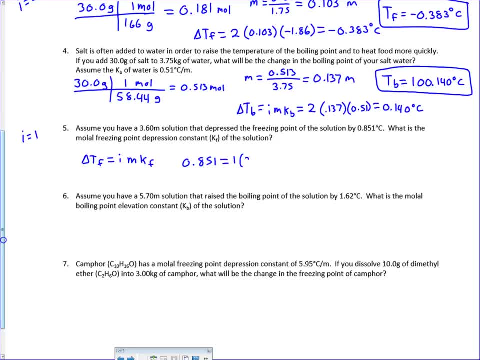 I. I said just assume that's 1,, the molality is 3.60,, all right, and Kf is our unknown here. so you solve there. you get Kf equals negative 0.236 degrees Celsius per mol-al. 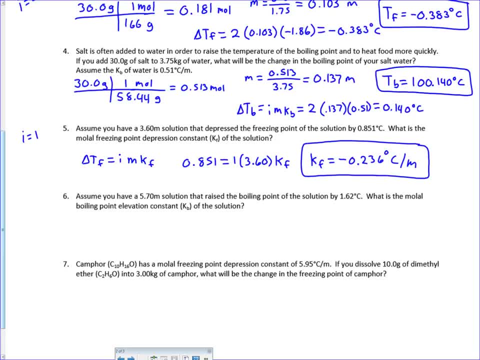 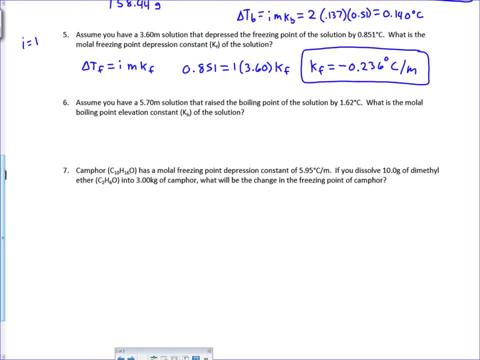 Number six. we're going to assume here again that I equals 1, because it didn't tell you what I was. So it's very similar, except this time we're dealing with the boiling equation instead. so you know, change in boiling temperature. 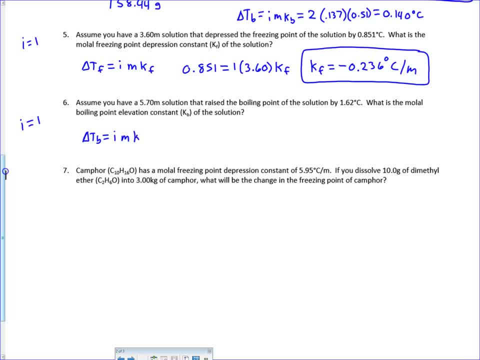 equals I times M times Kb- In this case it was 1.62- was our change in boiling temperature, which equals 1 times 5.70 mol-al. all right times our Kb. you solve that for Kb. you get Kb equals 0.284 degrees Celsius per mol-al. 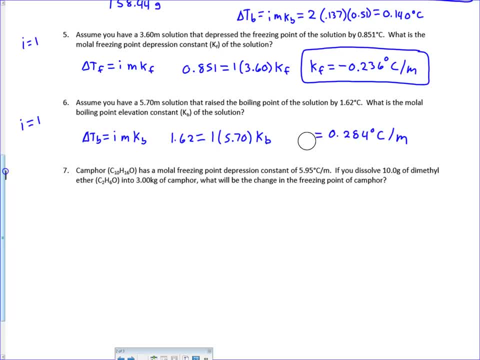 All righty. number seven. this one's a little bit longer. so it tells us: Km4 has a mol-al freezing point depression constant of 5.95 degrees Celsius per mol-al. so that's telling us how much the freezing point goes down. 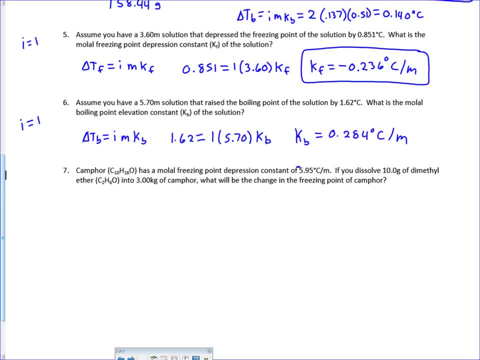 This should actually be negative here. all right, this should be a negative 5.95 degrees Celsius per mol-al 5.95, because it's how much the freezing point is depressed. So later on we'll plug it in that way. 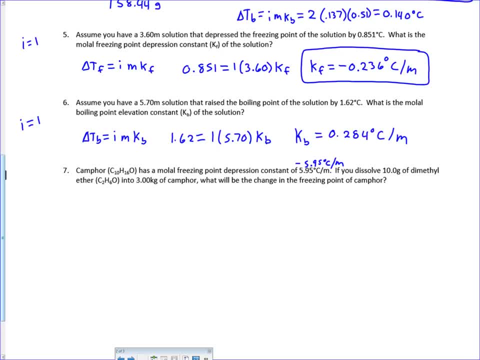 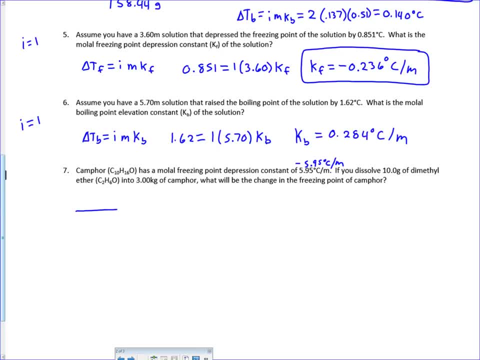 so we've got to get this to moles. to start off with, It says that we've got 10 grams of dimethyl ether, so 10.0 grams of C2H6O, And if you calculate that you get 46.08 for your grams. 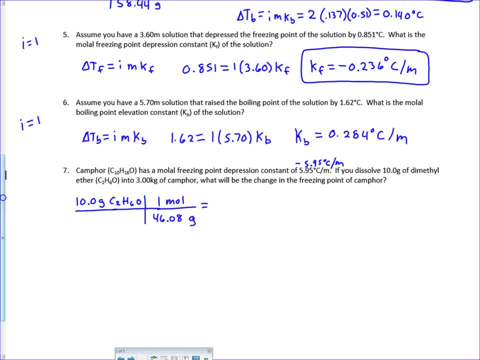 your molar mass for one mole. Calculate that you should get 0.217 moles of dimethyl ether. Then we can calculate the molality. Molarity is 0.217 divided by 3 kilograms, so divided by 3.. 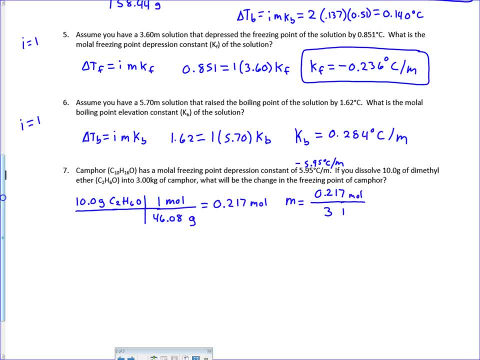 Which in this case equals 0.0723 molal. Then the next thing we've got to do, we've got to calculate the change in freezing temperature. So delta Tf here equals 1.. Okay, I'm going to say the Van't Hoff factor here is 1,. 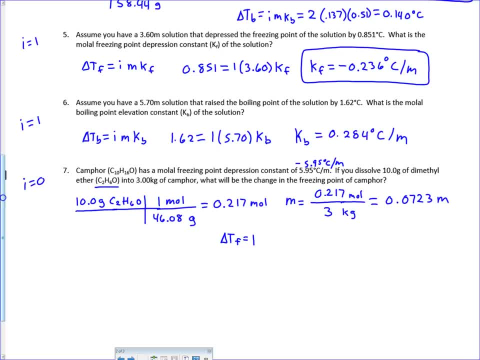 because our substance that we're dissolving here is this C2H6O, And all of that is non-metals, it's covalent, it's not going to split up when you put it into solution. So we're going to say I equals- oops, that should say I equals 1.. 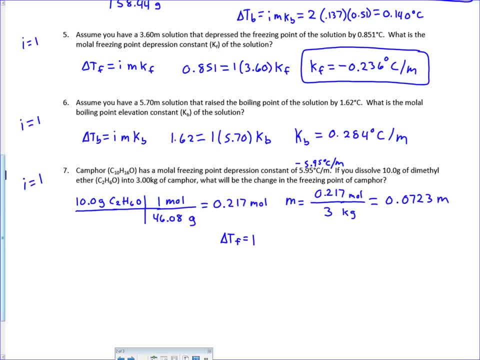 It's just going to be one piece when you put it in there. So I is: 1. The molality: 0.0723.. And then that constant there, that Kf of negative 5.95.. And I get negative 0.430 degrees Celsius. 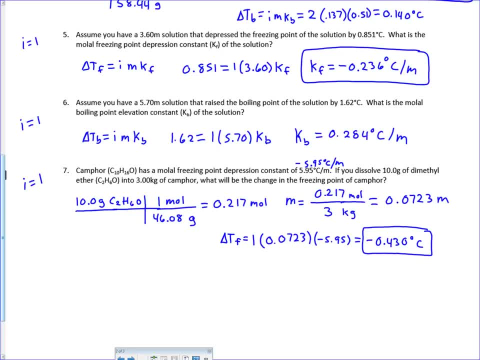 This is negative because it's freezing point depression. it's going to go down. We don't know the normal freezing point of camphor, but if you did, you would just subtract 0.430 from that. So let's say the freezing point of camphor was something like 40 degrees Celsius. 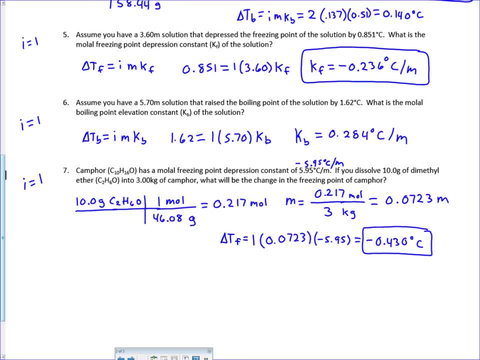 So 40 minus 0.43, that'd be 39.57,. okay, would be the new freezing point, And so you just take whatever the normal freezing point is, you subtract 0.43 from it. But again, in this one it just asked us for what the change was. 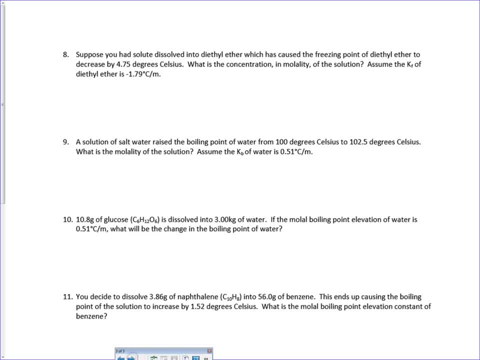 So this is our final answer here. Okay, just a few more problems here. left on this last page For number eight. here, what we've got here it says: you've got a solute dissolved into diethyl ether, and then it's asking us to find what the concentration is in molality. 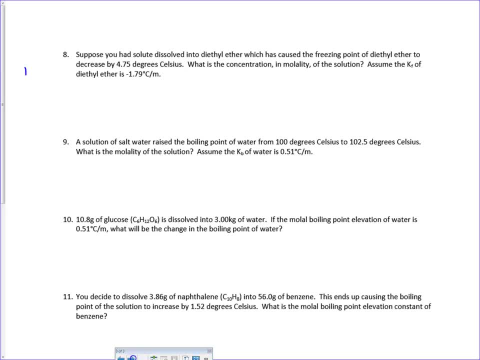 And so this is another one where they probably should have told us what substance we were having. They probably should have told us what the Van't Hoff factor is- I'm going to assume it's one- because they didn't tell us what substance we were dealing. 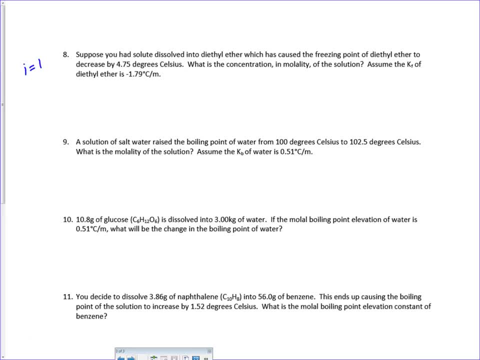 with here. So any time I don't give you a substance, assume that I equals one. So we know that the change in freezing temperature here is going to equal to I times M times KF. all right, And then the things that they gave you here. they told you that it changed by 4.75 degrees. 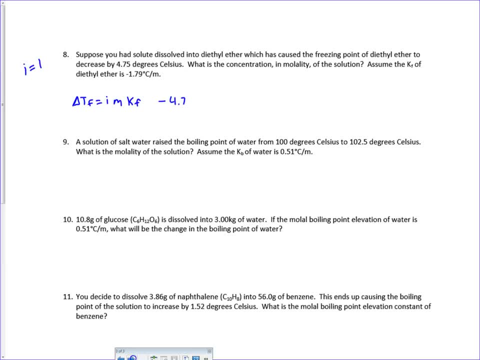 and since it was decreased, we're going to say negative 4.75 for our change equals Van't Hoff factor of one times our molality- that's what we're trying to find here- times our KF. It tells us there that the KF for diethyl ether is negative 1.79, okay. 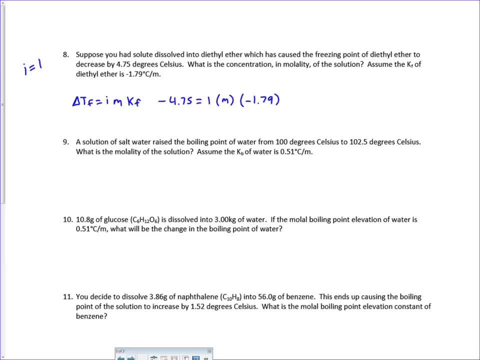 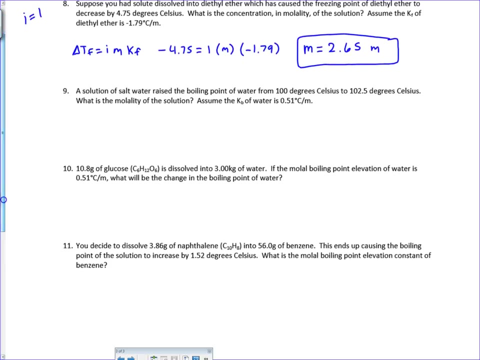 So you can solve this for M and you get that the molality is equal to 2.65 molal. All right, Thank you. Problem number nine here, Similar problem. what we're doing here, we're going to try and find the molality. 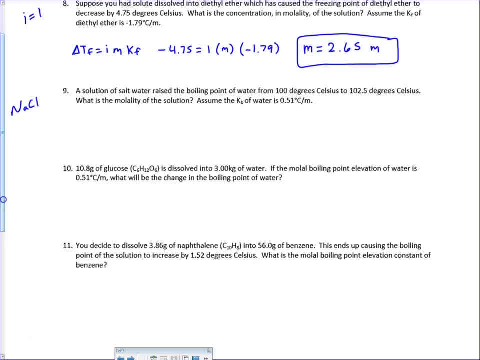 It's NaCl because it says it's salt water. so we know that I equals two. We're going to deal with the change in boiling temperature. equals I times the molality times 0.51.. Your boiling point constant, all right, so then we know 2.5, that's our change in temperature. 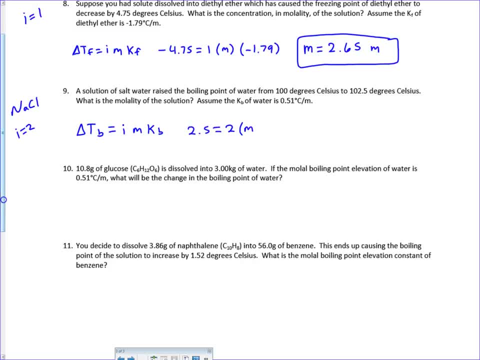 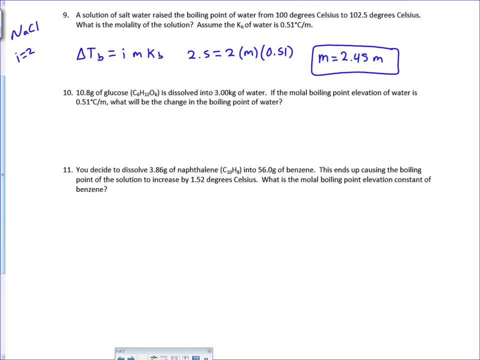 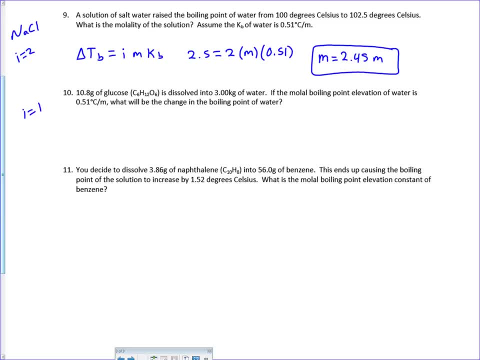 Thank you, All right, So what we've got here? we've got glucose. it says it's going to be dissolved Because it's glucose, that C6H12O6, all of those are nonmetals, it's a covalent substance. 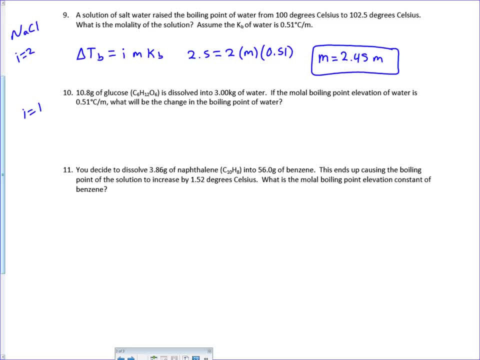 so it's not going to spread apart into pieces when you dissolve it. so for this one, I just equals one. It's asking us to find the new boiling temperature. so in order to do this, we need to figure out how many moles of glucose we have there. so we're going to start 10.8 grams of glucose. 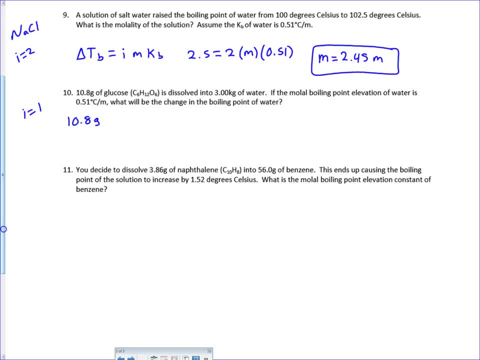 Okay, point eight: grams of glucose. The molar mass of glucose, if you add it up on the periodic table, is a hundred and eighty point one, eight grams for one mole. Multiply those together, you get zero point zero. five, nine, nine moles. Next we: 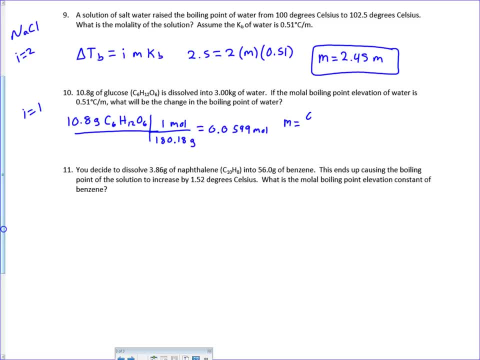 can calculate the molality. Molality equals that number of moles, zero point zero, five, nine, nine divided by the number of kilograms. In this case it's three, and that's going to give us zero point zero, two zero zero for our molality. Then we can plug it into the freezing point equation. So change in. 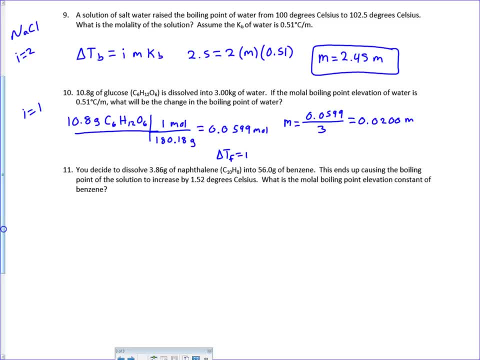 freezing point equals zero point zero. five. nine, nine moles Vantov factor: one times the molality point zero. two zero zero times the constant here for water. point five: one is our KF here, all right, and so I hope this is boiling point actually that we're talking about here, but yeah, point. 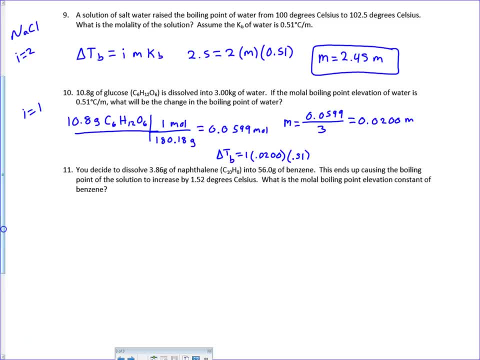 five one is what it is, so delta TB is actually what we need here. Multiply those together and we get zero point zero one, zero two. Now, since we're talking about boiling, the normal boiling point is 100 again, so the boiling temperature is going to be 100 plus that point. zero one, zero two. so I get 100 point zero one. 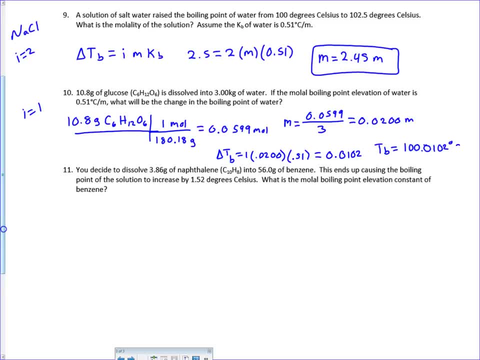 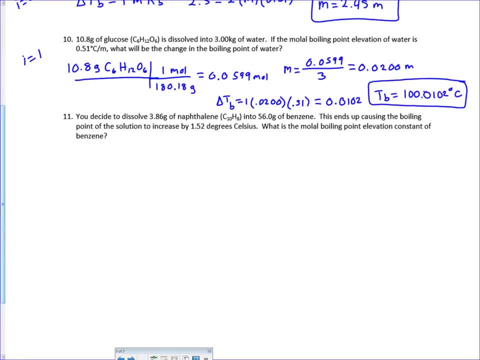 zero two degrees Celsius. Last problem here. So this one's technically talking about dissolving neptelene into benzene. So benzene is going to be our solvent here. Nephthalene is going to be our solute. We have to figure out how many moles of neptelene we 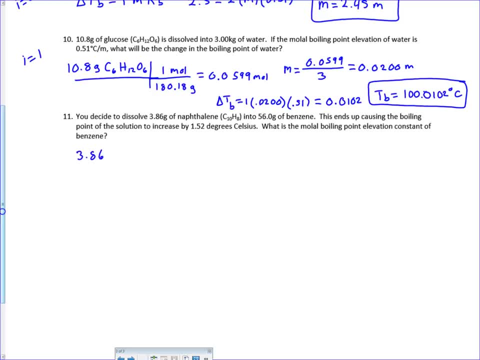 have Three point eight, six grams. The number of moles and the number of grams in one mole is a hundred and twenty eight point one eight. that comes from the periodic table. grams for one mole. Okay, go ahead and calculate that. you get zero point zero, three, zero one. 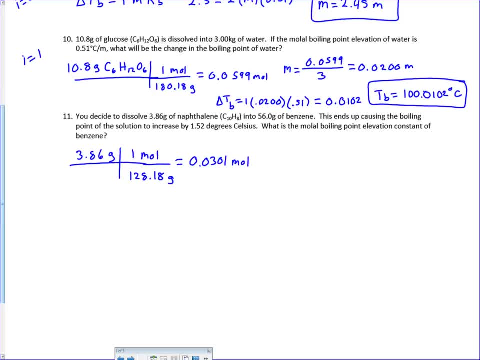 moles. Then we know the molality equals the number of moles. zero point zero, three zero one moles over the number of kilograms. This is, it's fifty six grams. so we gotta convert that to kilograms at zero point zero, five, six, zero. you calculate that you get zero point five, three, eight. for the 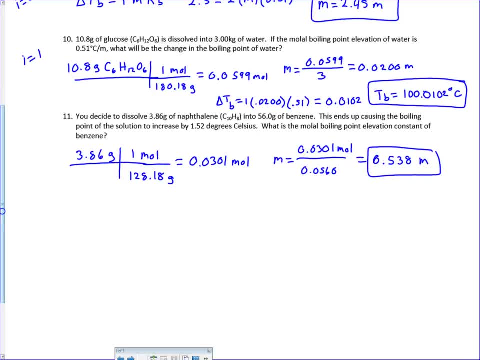 molality. Then we're to calculate the change in the boiling point. so change in temperature. boiling here equals times M times KB. Alright, we know 1.52 is our change in boiling temperature, because it told us that Vantoff factor, this substance, here C10H8, that is covalent, so the Vantoff 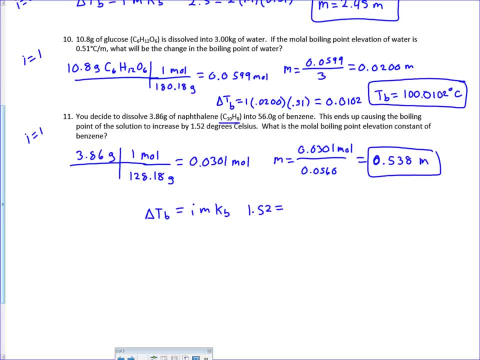 factor is going to equal 1 in this case. So 1 times our molality, 0.538 times our KB. Go ahead there, do the algebra, solve for KB and you get KB equals 2.83 degrees Celsius per molal. 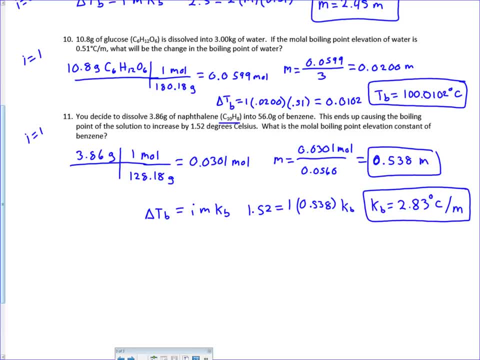 So I know that this is a long assignment and a long video. Lots of different ways. I can ask you questions about that. Just make sure that you understand all of this and there shouldn't really be anything other than this on the exam. So you know, make sure that. you're good with this and you should be good for the exam.